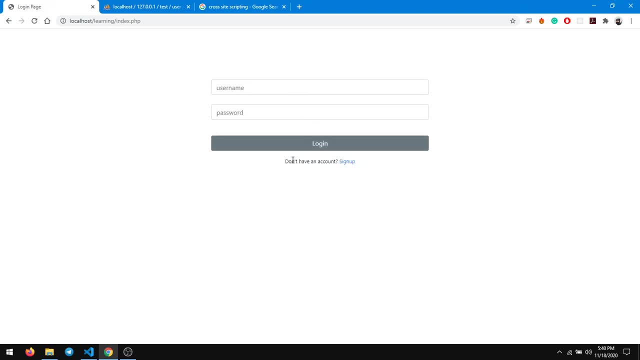 account, you can log in and you'll go to the dashboard and log out. So let me show you. Let's say I create with a name called Kira Kira, His name is Kira and the password is Kira and I click on sign up. When I click on sign up, it says: created account, please. 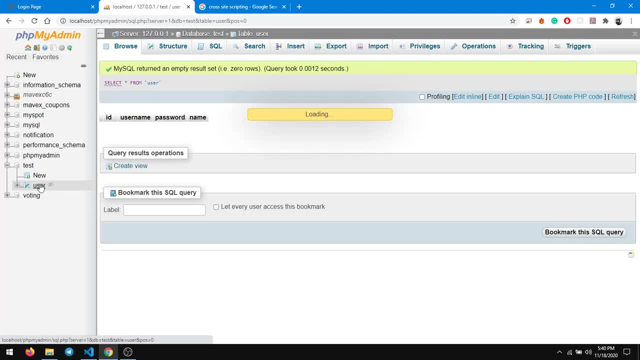 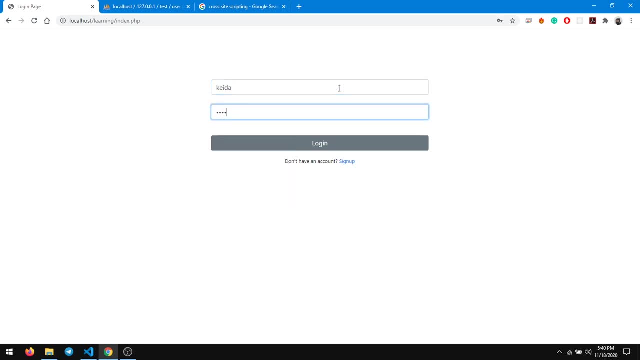 login and you can also check it right here in the database: Kira, Kira and the name is Kira. So if I log in with Kira and Kira and I click on login, it's gonna say welcome to dashboard Kira, Kira and I have a logout option. So when I click on 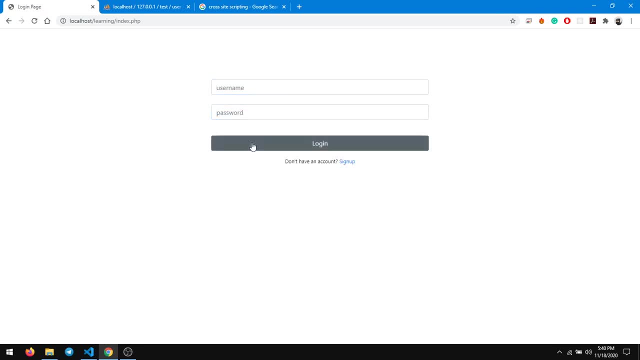 logout. i just come to the login page. Really cool, but what if I put my name as something like this: Ok, Look at it carefully. It's a script, Its JavaScript and what it is doing is locationhrefhttpsgooglecom. So this is script and executed, it will redirect you. 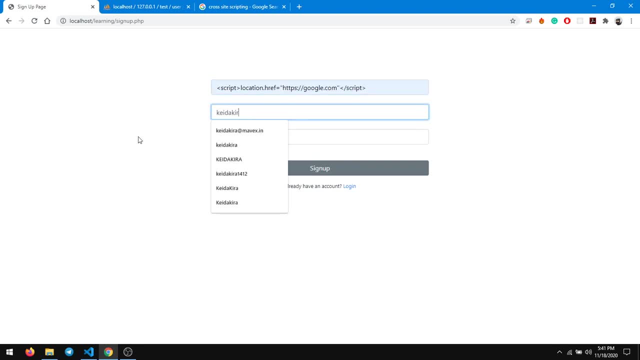 to googlecom And the username is KiraKira, The password is KiraKira. I'm just making a new account, So click on sign up It says create account. So I go to login- KiraKira, KiraKira- And when I click on login, just observe what's going to happen. 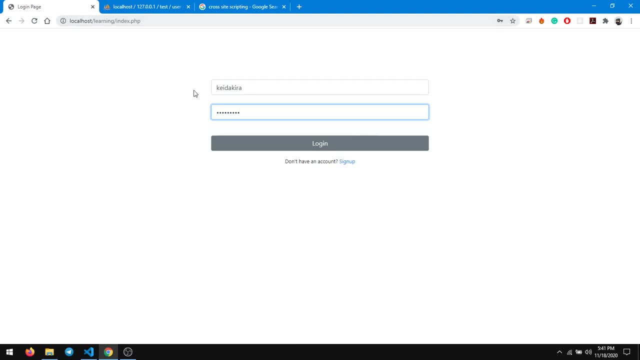 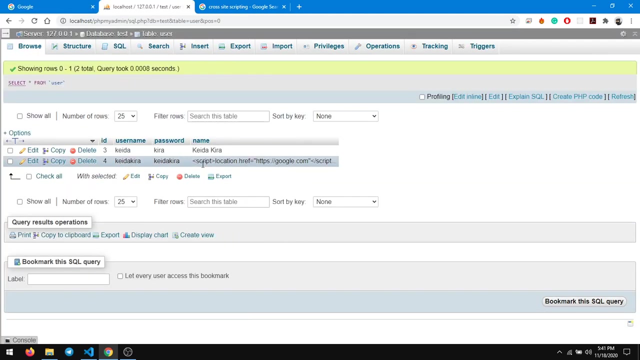 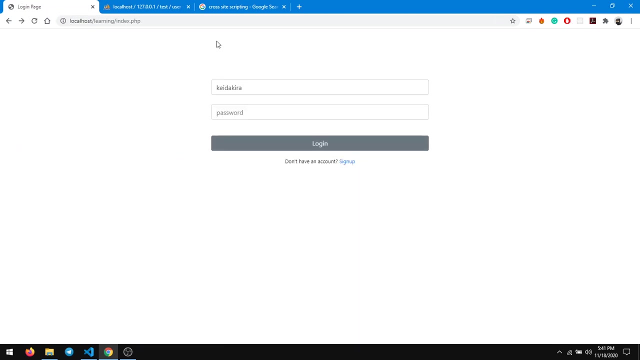 Okay, I'm presently on the indexphp page and I'm going to click on login. It has redirected me to googlecom. Why is that? Because if you check in the database, the name is stored as a javascript Right. So if I go to, if I log in again, KiraKira, But this time I'm 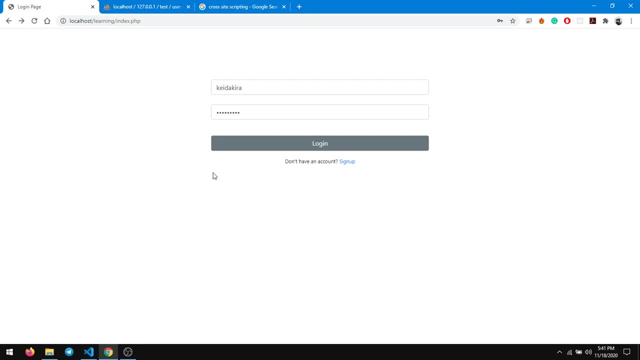 I'll be quick enough to go to the page source. So look at what's going to happen. Oh shit, I was not fast enough. Okay, So basically, what is going to happen is that script will be executed when you go to the dashboard again and again. 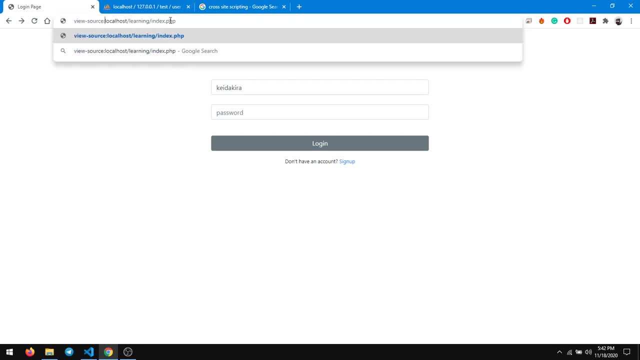 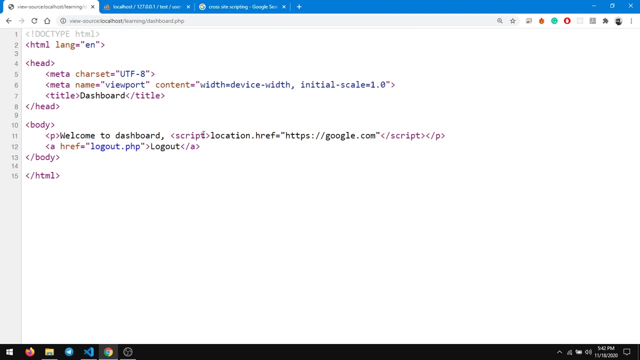 So if you now view page source, this is what is happening here. I'll go to dashboard. If you see it's it, Welcome to dashboard. And here it is executing a script. You see this, It's a javascript. It's colored, It's in. let me show you. Yeah, You see, It is colored in pink. That means it's a script, not a text. 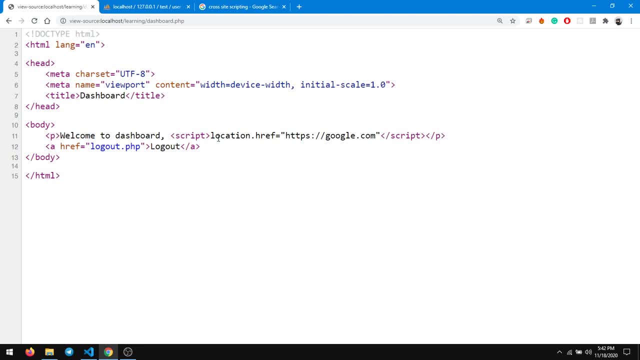 So, since it is a script, it will be executed. So this is what is known as cross-site scripting, So inserting a script in any input tags. It's the rough definition of cross-site scripting. So with this people can have a lot of problems. 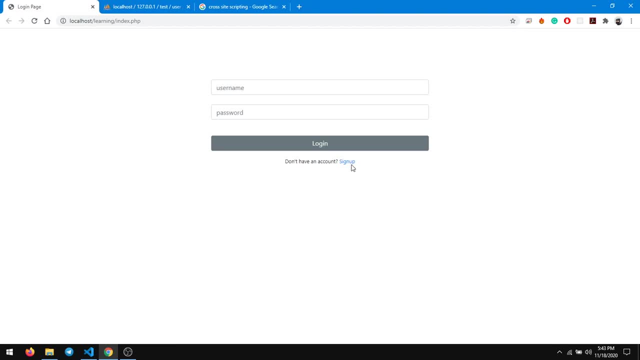 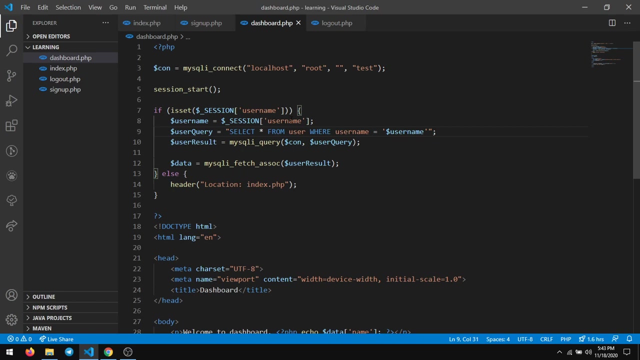 So how do you overcome cross-site scripting in PHP? You will overcome it using something called as HTML special cares. So we go to a dashboard page. The dashboard page has: I'll just explain the code very briefly, So you're just connected. 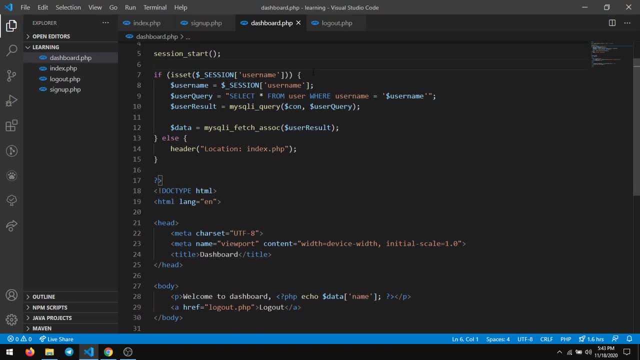 You're connected to the database, You start a session, which is pretty common, and you will check that the session is there. That means the user is logged in. If the user is not logged in, just redirect him to index page, which is the login page. 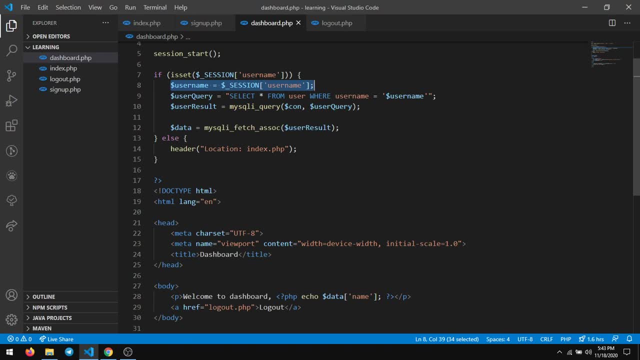 If he is logged in, we have the username stored in the session, So we extract the entire details with the username and we store it in user result, and we will extract the data using mysql-fetch-association array and store it in data. 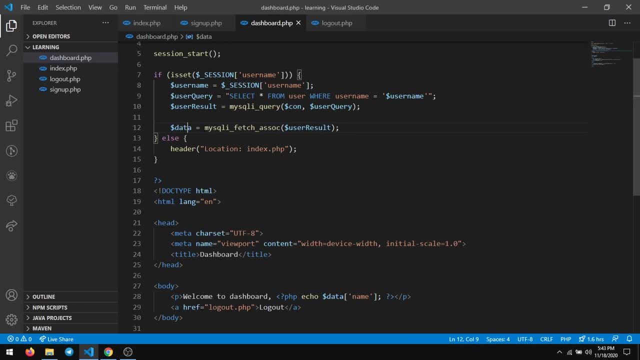 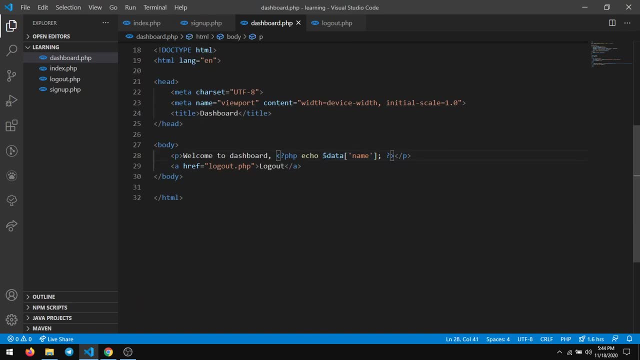 So data consists of his name, username and password, and that is what we are echoing here: the data of name. but here we will be encoding it and echoing it. So HTML- I'll show you HTML: special cares- okay, 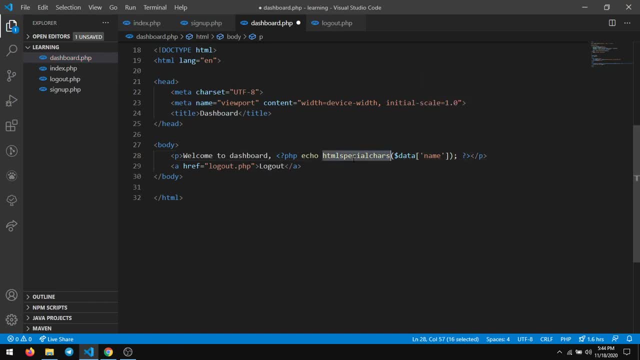 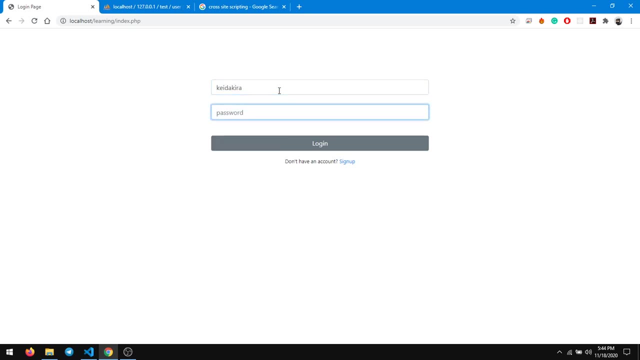 So, before echoing it, echo it this way. So I'm saving it and I'm Logging back again into the same account, Kira Kira, and I'm going to click on login This time. if you observe, we can see the script in the form of a text. 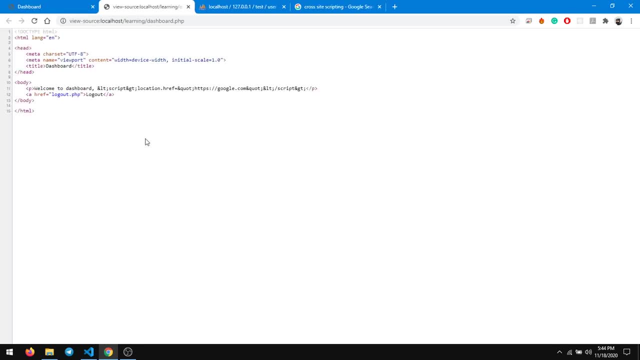 So if I go to page source, you can see that the less than is converted to ampersand LT, which stands for less than in HTML, and the greater than sign is converted to ampersand GT. So this way, even if the 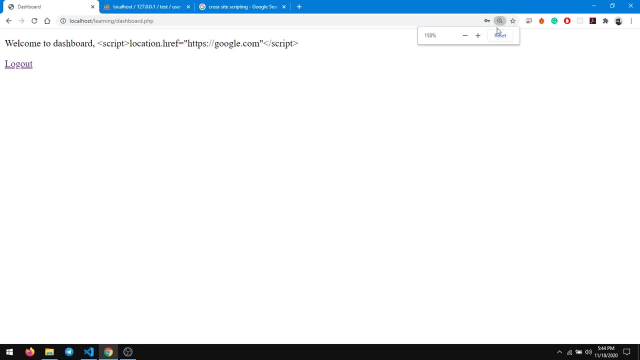 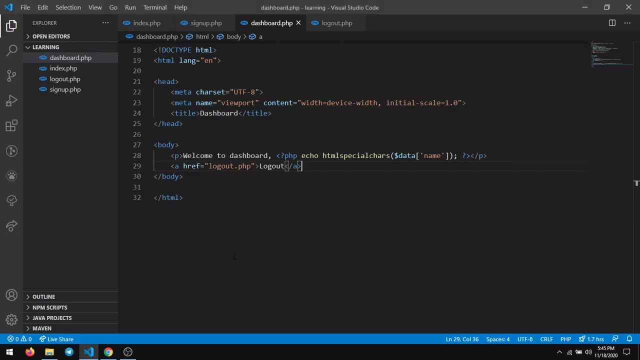 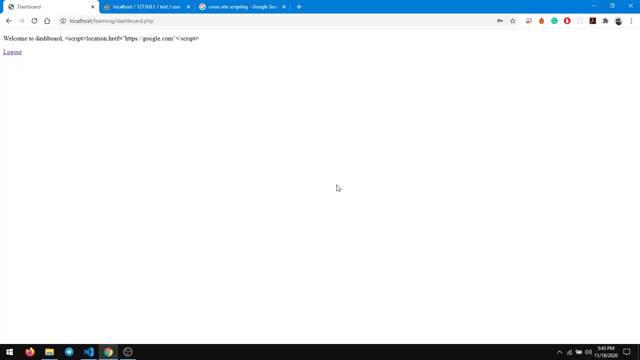 People who are hackers, of course, put different kinds of scripts, it will be disabled by PHP because of HTML special cares. So there are a lot of other ways, too, through which you can overcome this. One of the best ways is this: 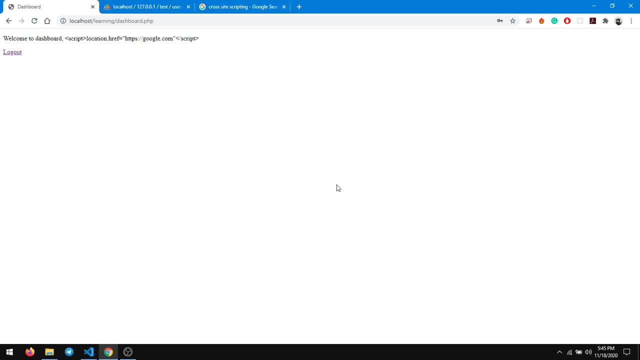 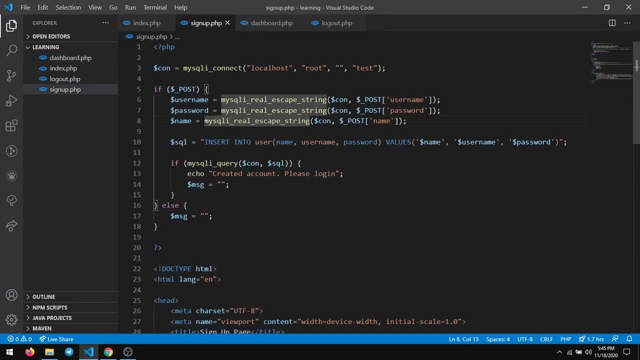 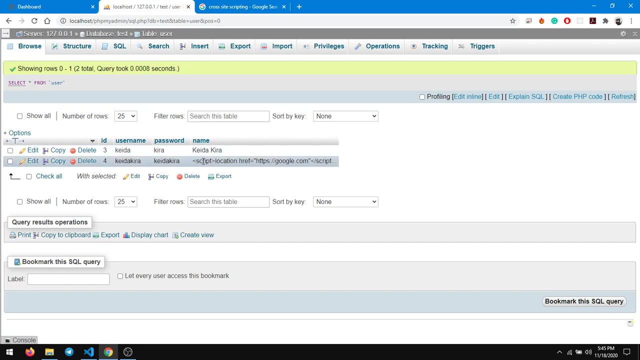 The other way is to directly encode it when you're inserting it to the database. So when you're inserting It into the database in the sign-up page instead of directly inserting the name here. if you check in the database, it is still stored as less than script. greater than location. 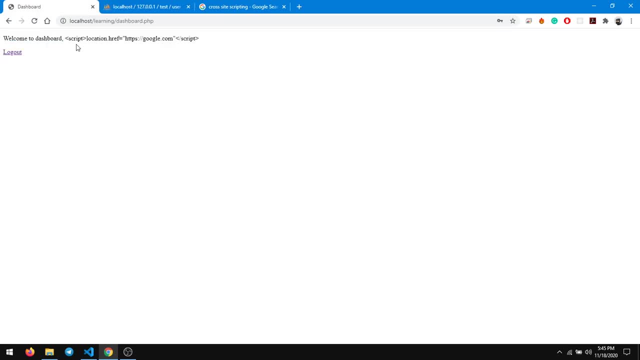 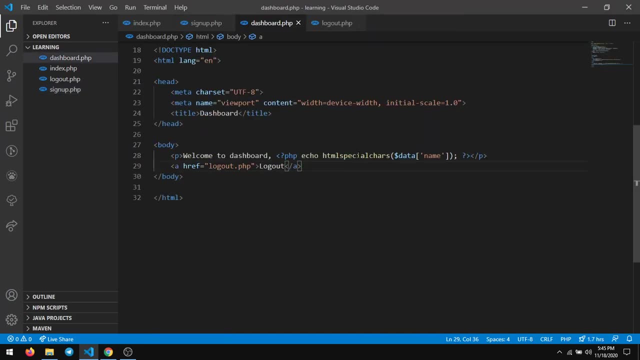 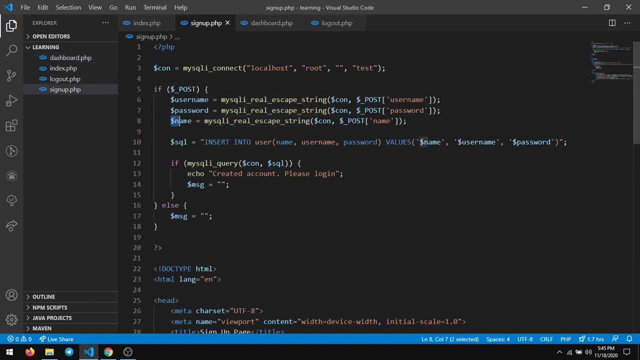 But what if we store here in this format itself? Then we don't have to write in HTML special cache every time we echo the data, Because if you forget it once then It's prone to XSS, right? So when you're inserting the data into the database itself, that is right. here itself you have to encode the data and insert it. 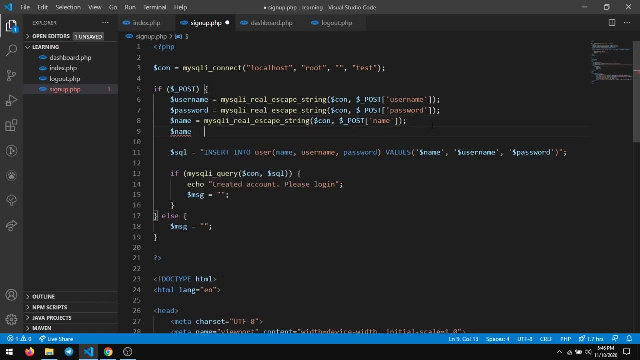 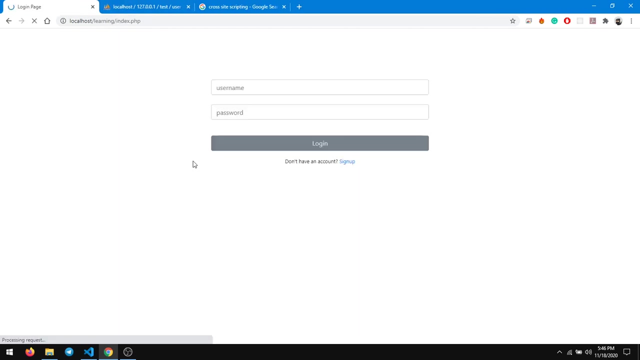 So how do we do that? Name is equal to HTML special cache. Yeah, Name. So this way you encode it and store it back into the name. So let us sign up now. Again, We'll use the same script. 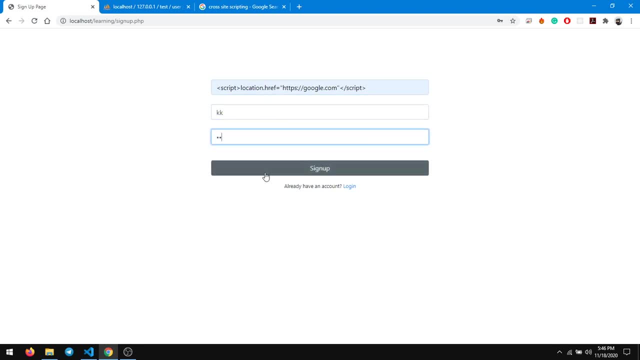 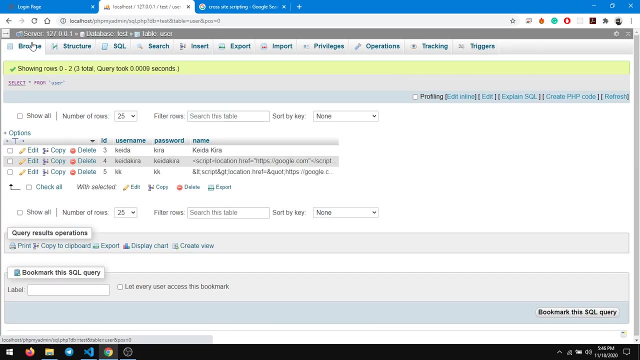 And let's say KK, KK And we'll sign up, And now we are going to log in back again. But if you check in the database you can see that in the database it is stored as less than. The less than is stored as ampersand: LTCemicode. 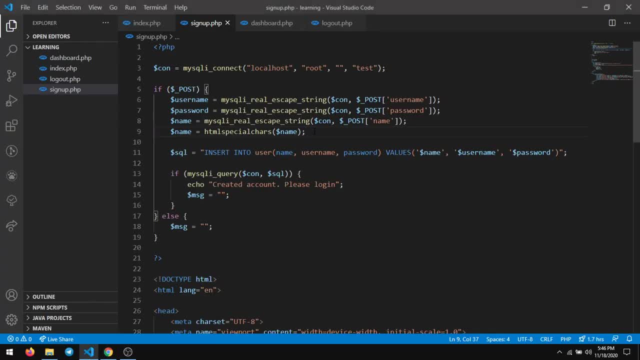 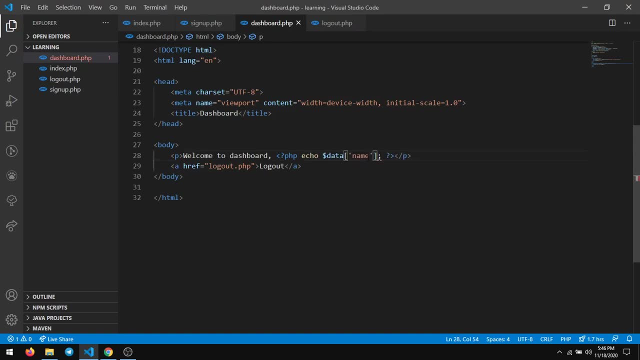 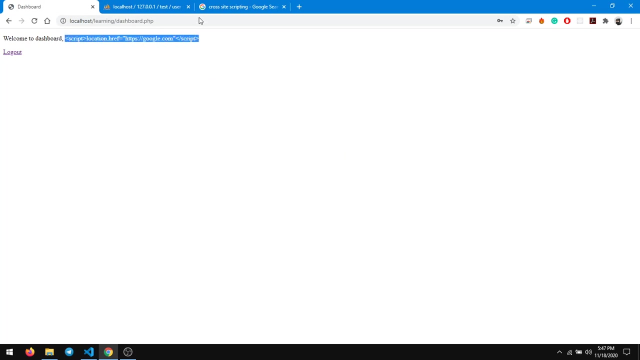 So this way you don't have to use HTML special cache every time time you're echoing, so I can just remove it here and keep it like I used to previously and I log in. you see it's working. so these are the two ways in.